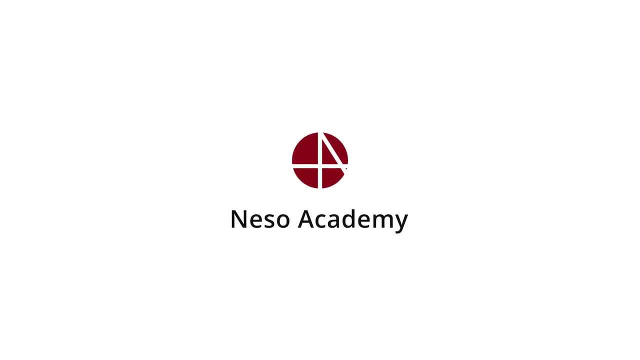 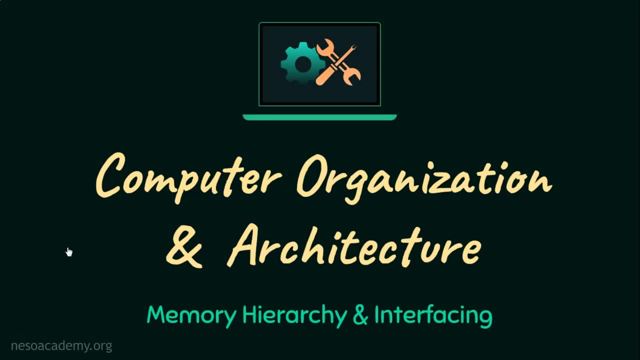 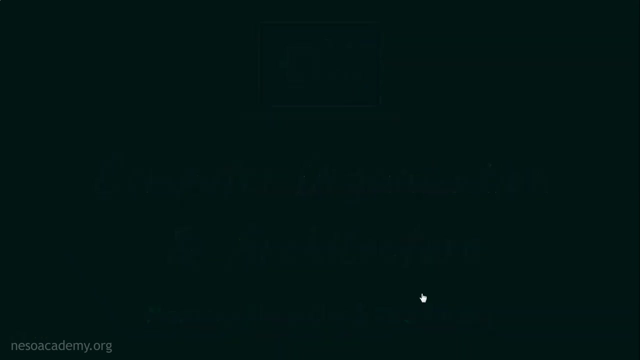 Hello everyone, welcome back In this session. we are going to learn about first the memory hierarchy, and then we will have a brief introduction regarding how the different memory units are interfaced with the processor. So let's get to learning Now. the term hierarchy, if put. 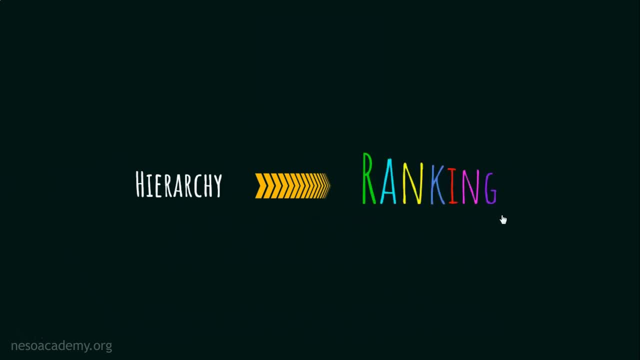 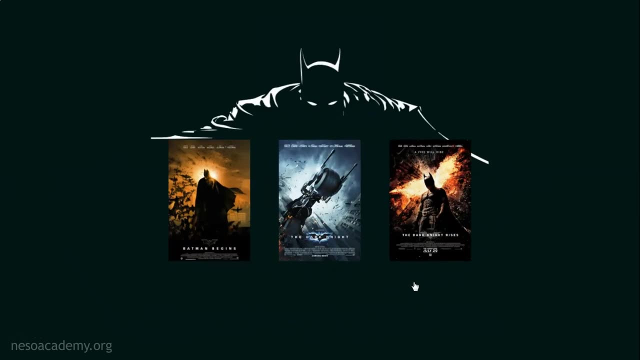 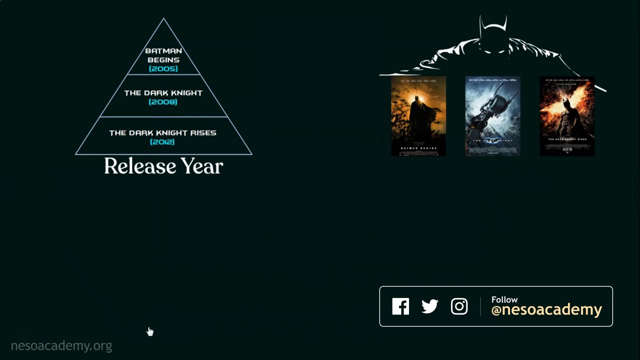 simply means ranking. Also, ranking can be done based on different parameters. For an instance, if we consider Nolan's Dark Knight trilogy according to the release dates, Batman Begins comes first, then the Dark Knight and finally the Dark Knight Rises. But if Rotten Tomatoes, 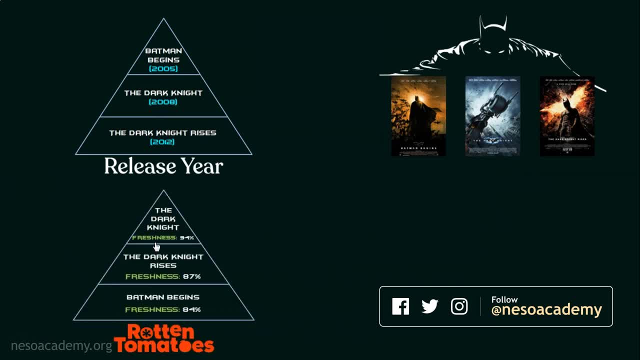 Tomato Meter is considered, the Dark Knight is on the top, having the freshness of 94%, Because, honestly, Heath Ledger just rocked it right. Then comes the Dark Knight Rises and finally, Batman Begins. Now, this ranking remains the same if Metacritic scores are also considered. 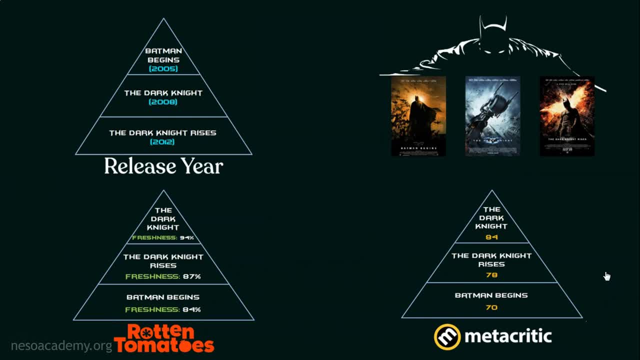 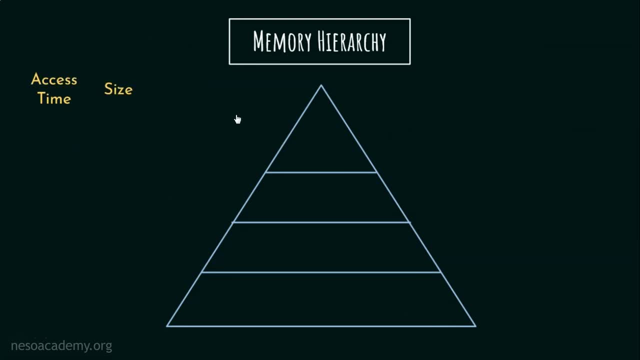 Similarly, based on different aspects, the memory storages can also be ranked. If we consider access time and size, we can rank the memory units like this. Registers are made up of flip-flops and are embedded within the processor itself. Therefore, time to access them is the least. 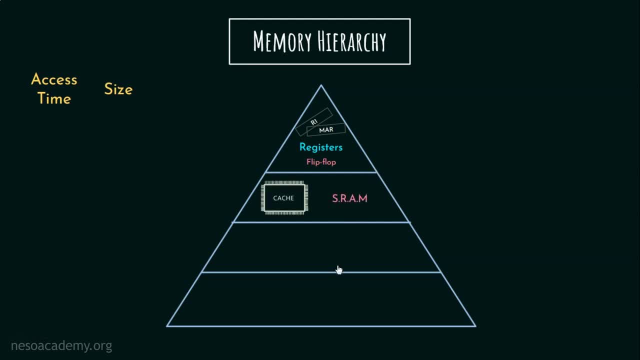 The SRAM caches are next followed by the DRAM main memory, last but not least, the secondary memory storages. However, in terms of cost and usage frequency, this hierarchy is reversed. I mean, as we move up in this, the cost and the frequency. 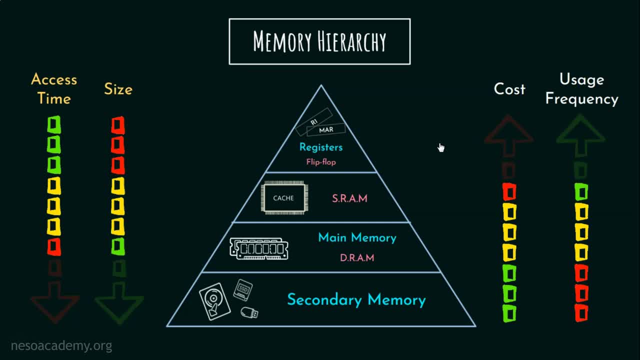 of usage increases. In our previous discussion we already understood that the processor is very fast and the sole purpose of having the memory hierarchy is to bridge the speed mismatch between the fast processor to slow memory. that, too, at a reasonable cost. Now, 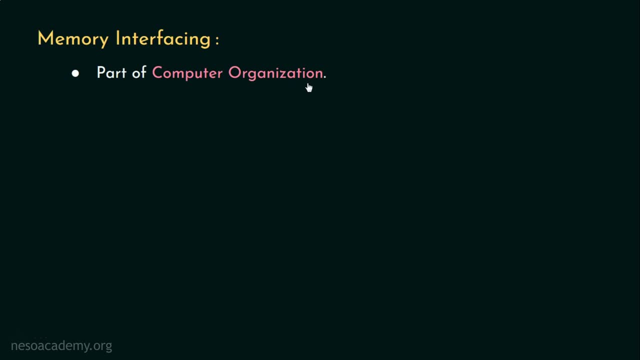 coming to memory interfacing, It is a part of computer organization which deals with the way of connecting various levels of memory units, especially to the processor, also to the I-O peripherals. Generally the speed of the processor is counted using the unit MIPS. Some call it MIPS. It stands for Million. 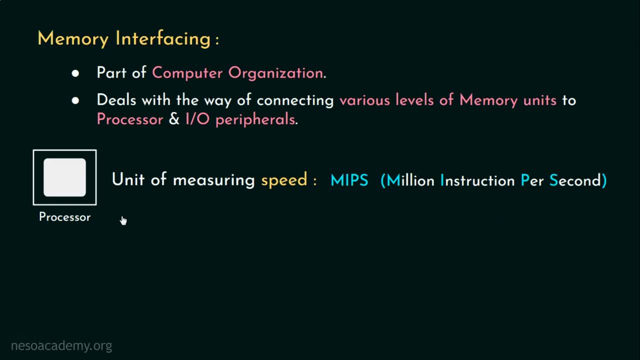 Instructions Per Second And our goal is to try to feed the processor with those many instructions from the memory in a faster yet cost-effective approach. Let's try to understand various levels of the memory. If I say information at nth level is a subset of the information available in the nth plus 1th level, it means if the processor 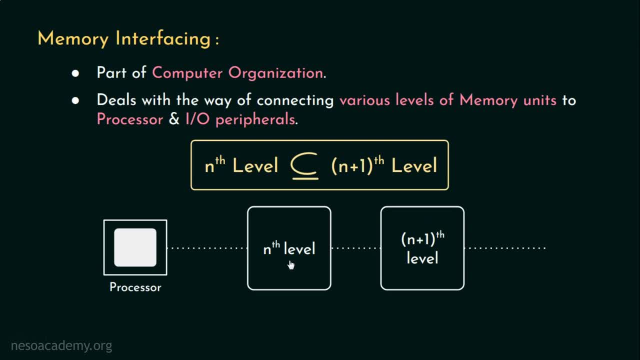 refers to the nth level memory for something. may that be any instruction or data? if that's found there, only we term it as HIT, Otherwise it's called a MISS, and the processor then goes to the nth plus 1th level, that is the next level to look for the same. So in case 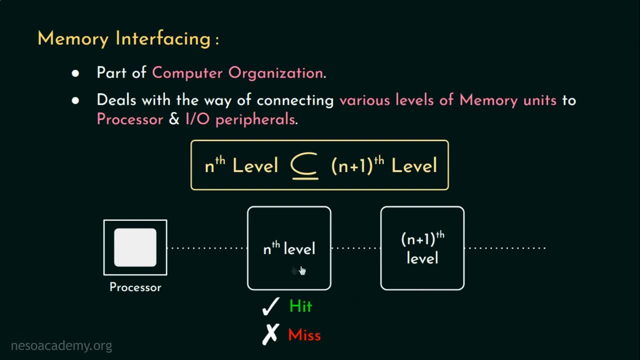 of MISS. the time taken to look for the information in both nth level and nth plus 1th level should be considered. However, it's not always the case. It actually depends on the way the interfacing has been done. Let's dig a bit deeper Now. generally, interfacing is done in two ways. 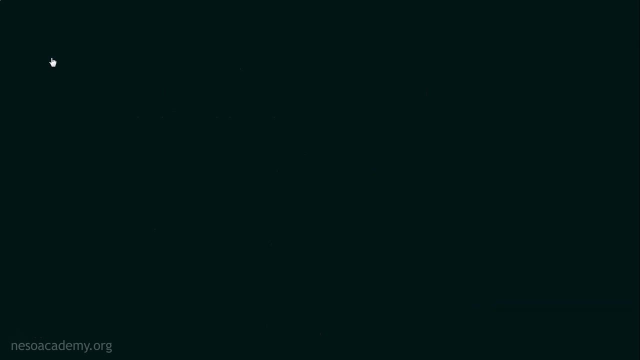 The following illustrations will help us understand these ways. Way 1. All the different memory levels are simultaneously connected to the processor, and whenever the processor wants some information it can be connected to the processor, So we can look for it in all the different levels side by side. Here the processor is connected. 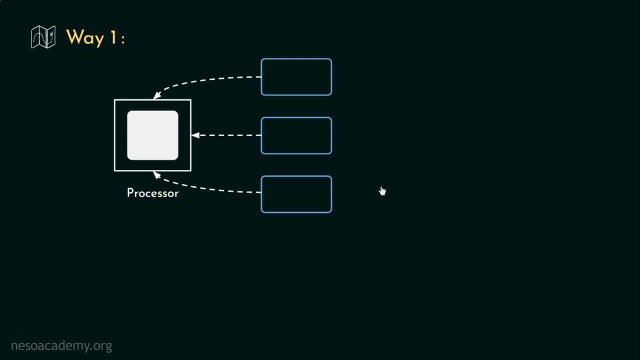 to three memory units of different levels. Now, for the time being, let's call them M1, M2 and M3.. Assuming the access time for these are T1, T2 and T3.. Also, T1 is less than T2,. 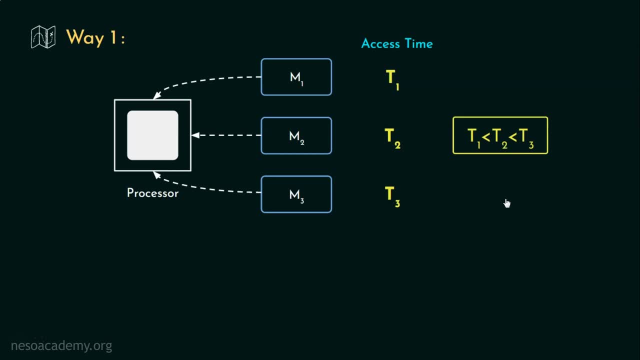 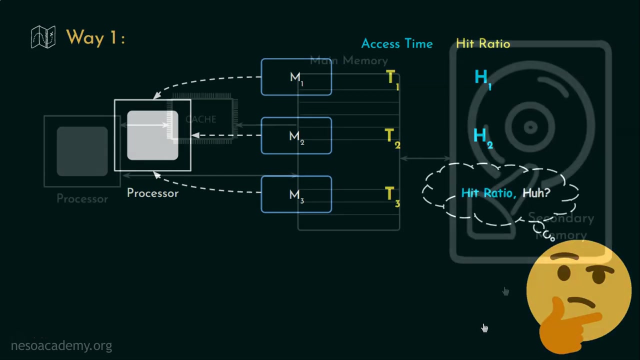 which in turn is less than T3.. Now let's presume that for a program or a set of instructions, the hit ratio of the M1 and M2 are H1 and H2.. All right, now the question that you must be having is what on earth is hit ratio right? 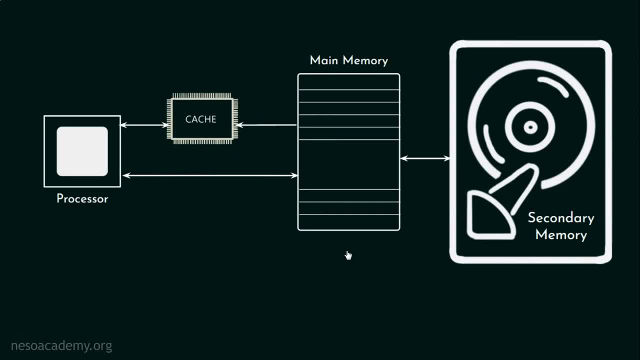 Now we already know that during execution the set of instructions are brought into the main memory from the non-volatile secondary storage. Also, the frequently accessed portions are stored inside the cache. Let's just say there are 100 instructions in a program and 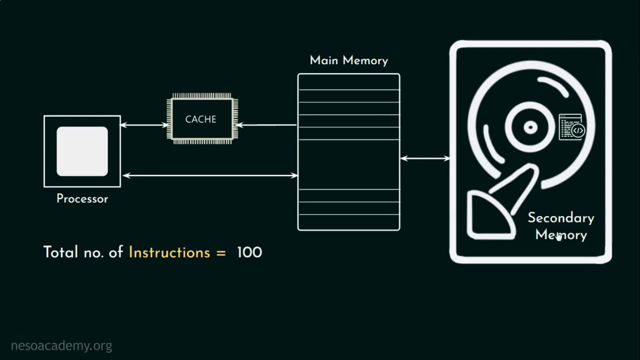 it's permanently stored inside the last level of memory hierarchy, that is, the secondary memory. Suppose from those 100, 80 of them are brought into the main memory. In that case the hit ratio would be 80 by 100, that is 0.8 or 80%. This means during execution there is 80% chance for the processor. 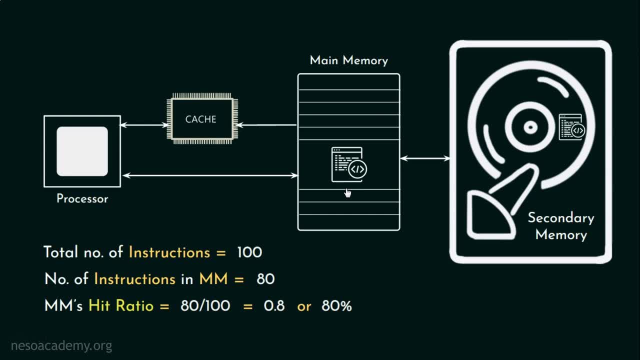 of getting the required instructions inside the main memory. Now, as the last level is nothing but the permanent storage there is, the hit ratio is naturally 100%. So we don't really bother about it, because if the program isn't there, there is no way for the processor. 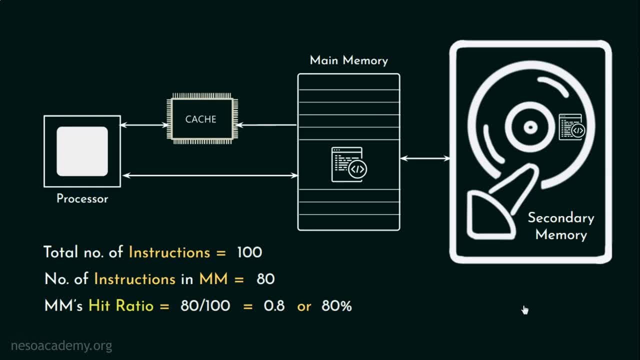 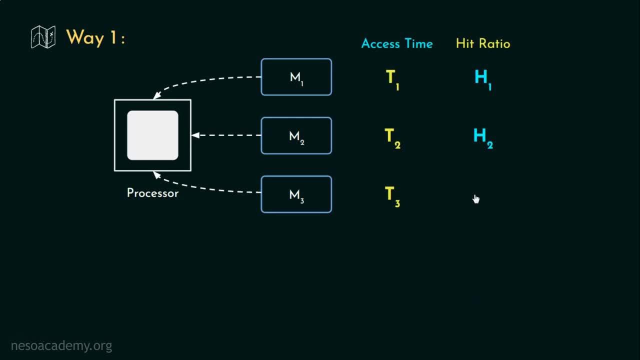 to execute it. It's like if we don't really have the audio file, how on earth we can play it? So, coming back to our illustration with all these informations, if we now try to find out how much time is needed, on an average, to find out an information in this organization, 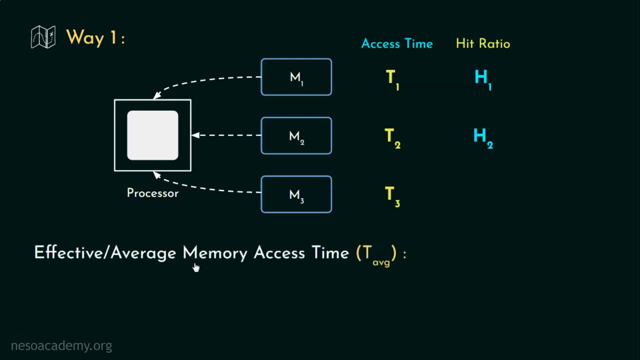 which is, by the way, popularly known as effective or average memory access time. the formula is as follows. Let's understand this formula so that we don't really have to memorize it. So there is h1% chance of finding the input data. 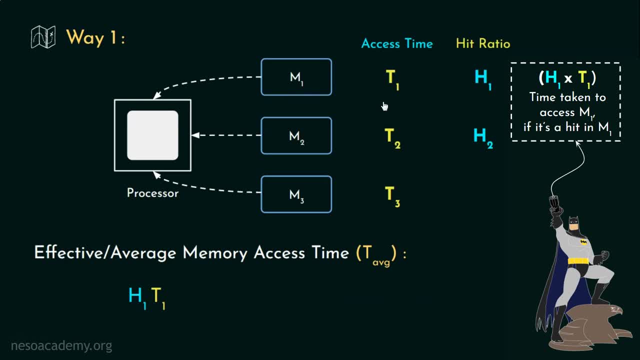 the instruction inside M1 and this is the time taken to access M1.. Now, 1 minus H1%. chance is also there that the processor may not find the instruction required inside M1, which is called the miss rate or miss ratio of M1.. 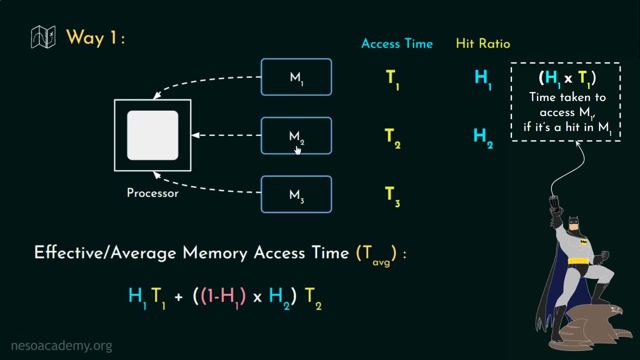 For those cases the processor will look inside the next level, that is, M2, which has H2% chance of having the instructions in it. Also, the time taken to access M2 is T2, hence 1 minus H1 multiplied by H2 and T2.. 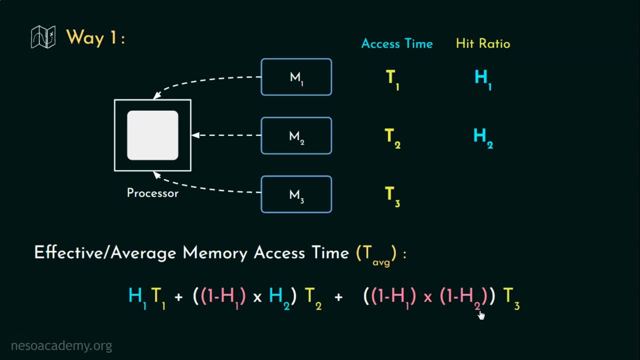 So finally, there are 1 minus H2% chance of not finding the instructions inside M2. that is, the miss ratio or the miss rate of M2 is 1 minus H2.. Therefore, 1 minus H1 multiplied by 1 minus H2, that is considering all the chances where 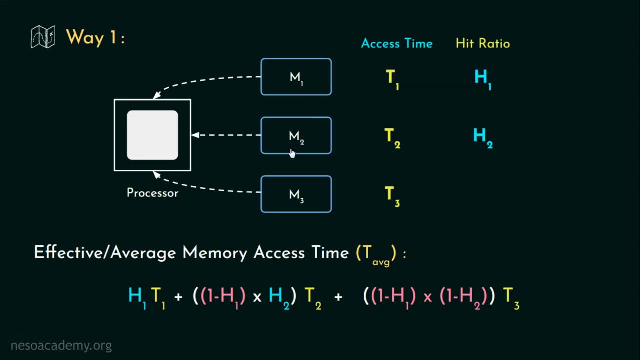 we can't find the required instructions either in M1. Or in M2.. In that case, we will have to look for it inside M3, that is the last level, And the time required to access M3 is T3.. Hence 1 minus H1 multiplied by 1 minus H2 multiplied by T3.